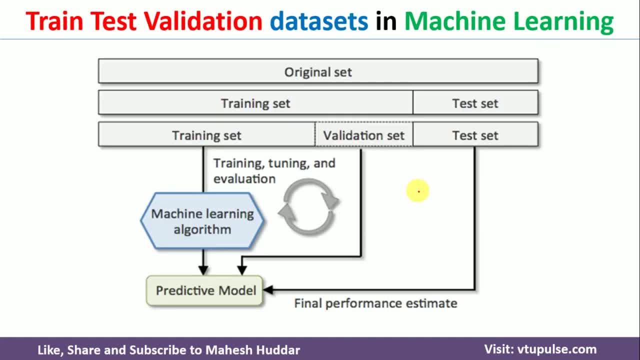 of testing set. The extended version of this particular model is something called as a train test validation. In this case, again, the original data is divided into training and testing set. This training set is again divided into two parts: the training and validation set. here, With the help of training set, we will train our model Once the training is. 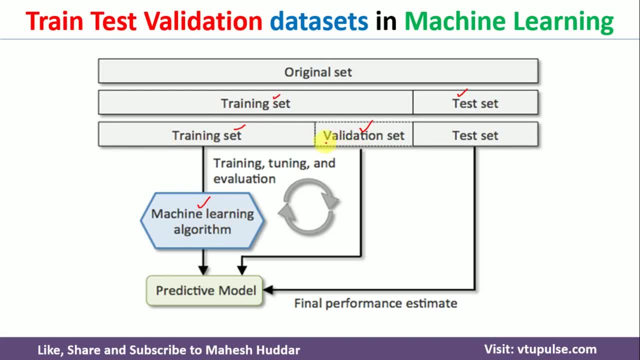 over. we will see the performance of that particular model with the help of training set. If we are happy with that particular performance, we will go with testing of that particular model. If the performance is not satisfactory, the model is tuned with the help of different hyper parameters and so on, And then again we will validate that particular. 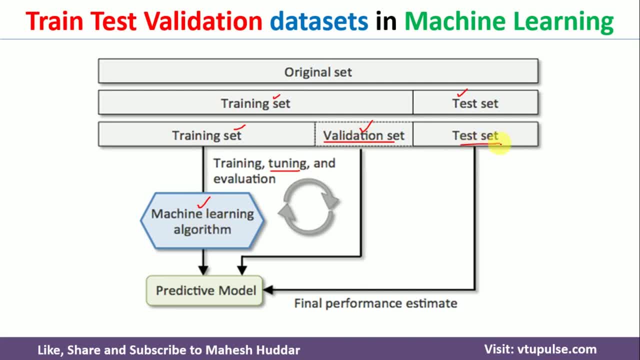 model. Once the validation is over, we will test it with the help of testing set here. Once the testing is over, based on the performance, we can deploy that particular model in real world, or else we can do some hyper parameter tuning And then we will test it again at the later stage. But in both this particular techniques, 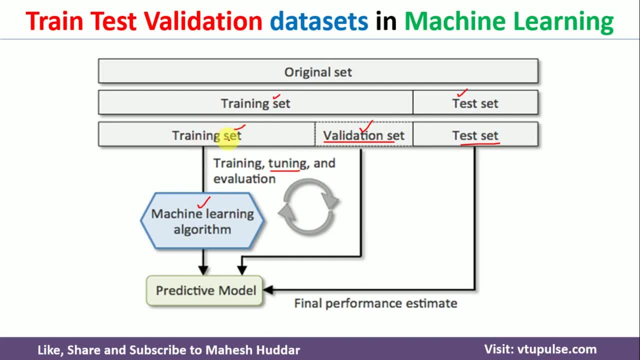 what we do here is we will take one part of that particular data as a training, another part for validation and the third part for testing. here, And if you follow this particular approach, there is a bias in this particular model, because certain part of the data is. 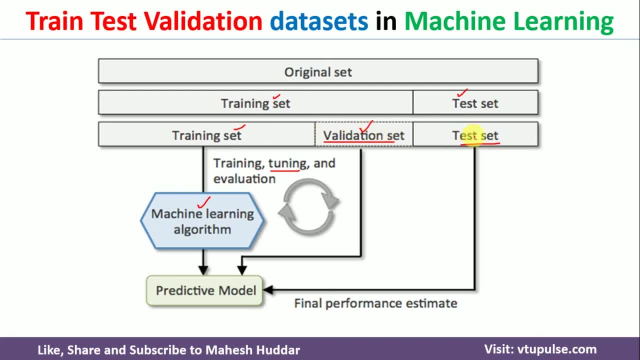 used for training. certain part of the data is used for validation and remaining is for testing over here, So the model is not trained or tested with the entire training set there. These are some of the best practices that we have misunderstood in this particular model. 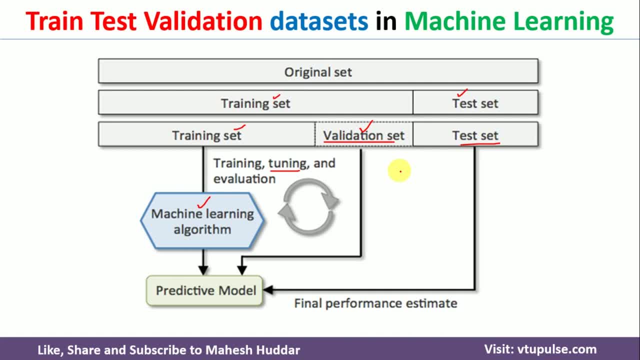 the data's representation over here. because of that, the model may go into something called as overfitting state here, that is, the model will work perfectly on the training data, but it will not work on testing or it may not work as expected in the real world over here. to avoid these, 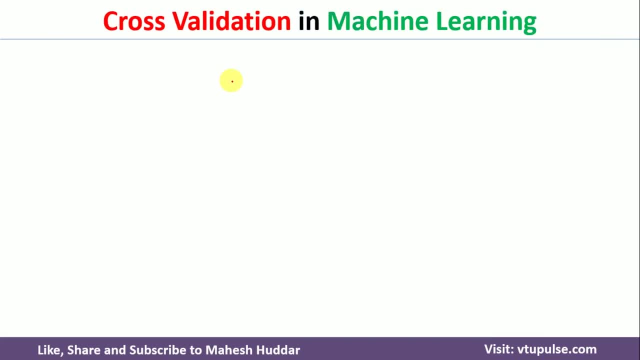 particular difficulties, we come across something called as the cross validation. in cross validation, what we do is we will train the model with the entire data set as well, as we will test that particular data model with the help of entire data set over here. so before we understand the 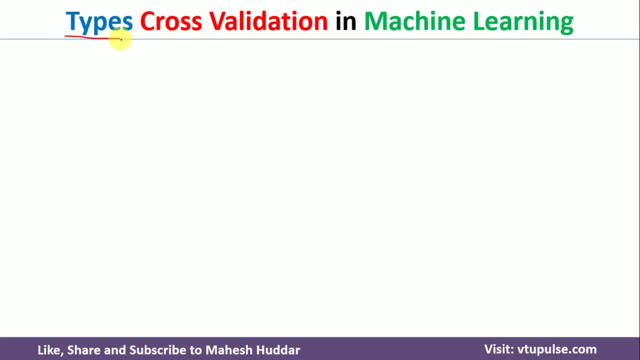 cross validation. we will try to understand what are the different types of cross validation. we have the very first cross validation, what we have is called as the keyfold cross validation. second one is stratified keyfold cross validation. third one is leave one out cross validation. fourth one is leave p out cross validation. we will try to understand each of these particular. 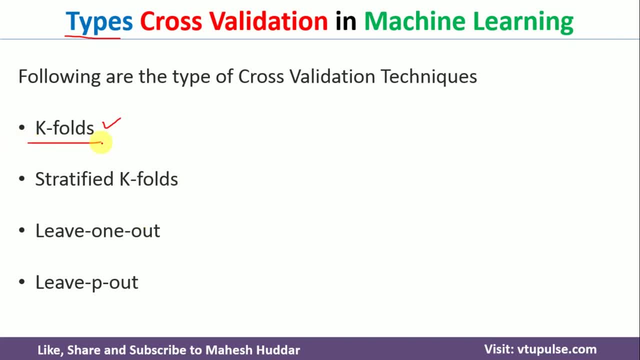 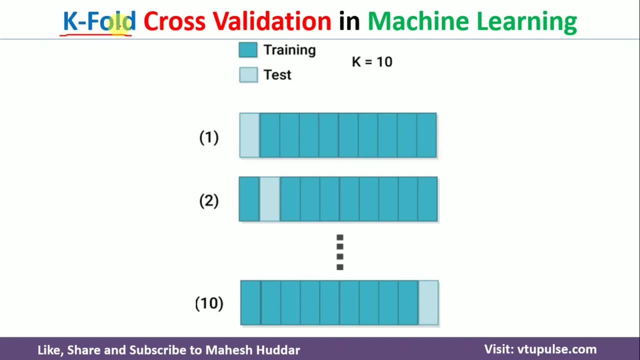 techniques one by one. first we will train the model and then we will continue with the keyfold cross validation. in keyfold cross validation we will divide the entire data set into k folds. that is, let us say that we have the k value is equal to 10 here. so the entire data is divided into 10 folds. you can see here, this is the first. 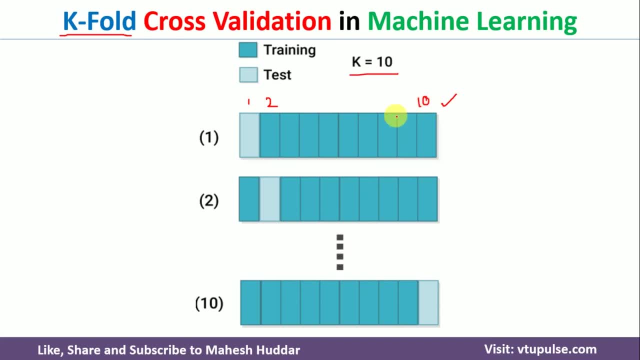 one, this is second one, and so on. this is the tenth one in this case, and we will train this particular model 10 times over here, because the value of this particular k is equivalent to 10 in this case. and now we will step to� the path serves, where we take the community, and then we will take the team performance and we will 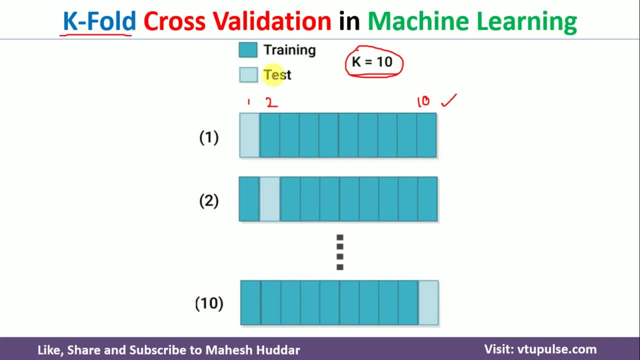 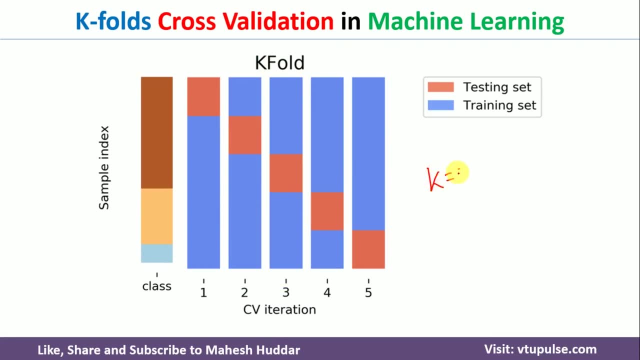 able to understand what the data is. that would be all of these elements are taking all this into consideration, performance of this particular model. here, To understand k-fold cross-validation, I will take one more example. In this particular case we have set the k is equal to 5. here The meaning: 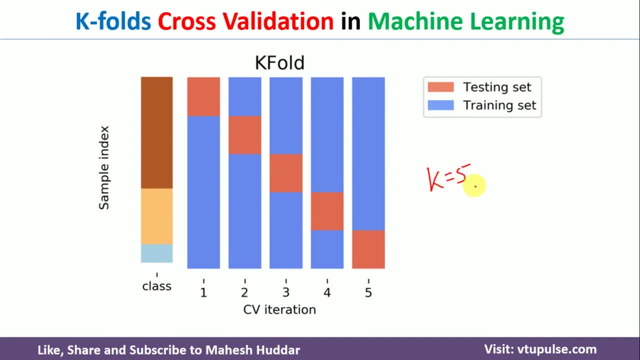 of this one is we want to divide the data into 5 folds In each and every iteration. we want to take one fold for testing, remaining 5 folds for training over here. So if you look at this particular first iteration, this particular thing was used for testing and this remaining 4 folds. 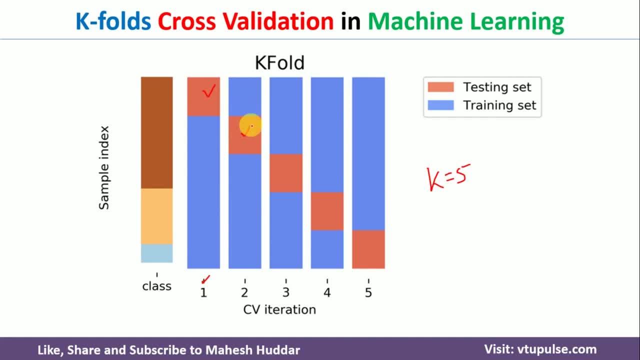 were used for training. in this case, In the second iteration, the second fold was used for testing. remaining 4 folds were used for training and so on. But k-fold cross-validation has some disadvantages. Let us assume that we consider this particular class of that particular data. 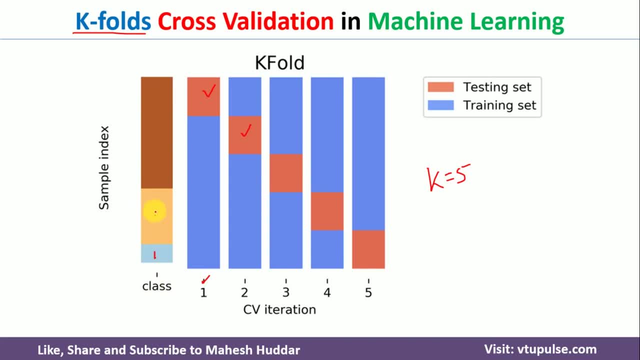 In this particular data set we have 3 classes. This is the first one, and this is second one, and this is third one. And if you look at this particular 5 iterations, in the first iteration the first fold, that is, the testing fold, is coming from this particular 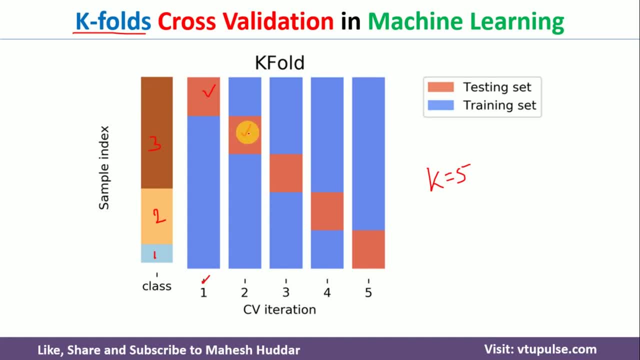 third class of this particular data set. In the second, again, it is coming from this particular class and in the last one it is coming from first and second class over here. So the meaning of this particular thing is in each and every iteration we are not taking equal representation of each. 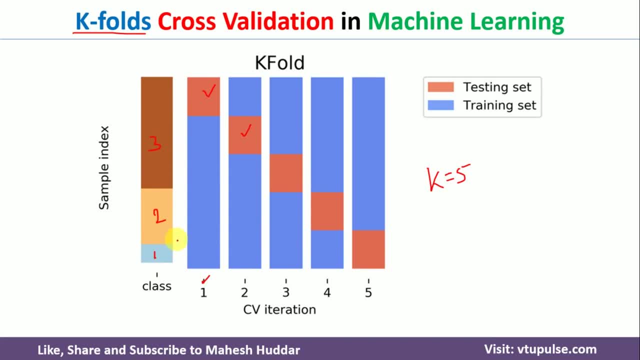 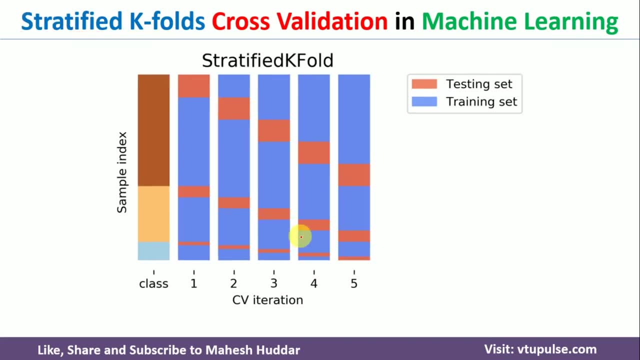 of these particular classes over here. Because of that again, it may go into something called as the overfitting state over here. To avoid this particular thing, we use something called as the stratified k-fold cross-validation In this case. what we do here is: 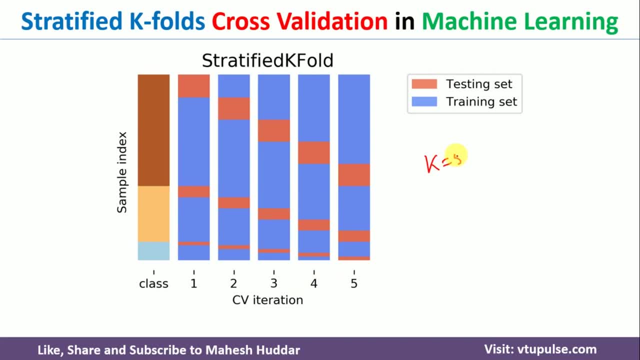 rather than dividing that particular data into 5 folds, we will divide that particular data in such a way that each of these particular folds will have equal representation of this particular classes over here. If you look at this particular first iteration, you can see here this particular. 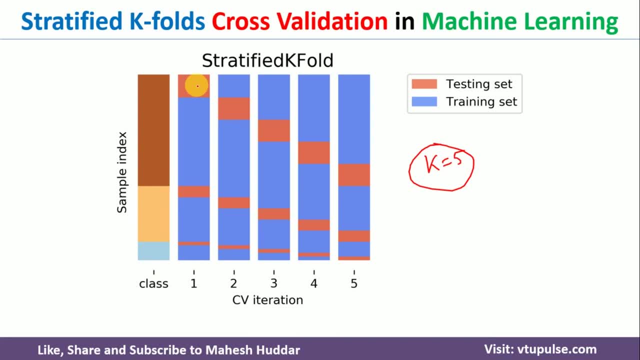 thing which is represented in a red color. this is a testing fold and it is having equal representation of each and every class over here. This is what the representation for each of those particular classes. The same thing has happened in the second iteration. third iteration. 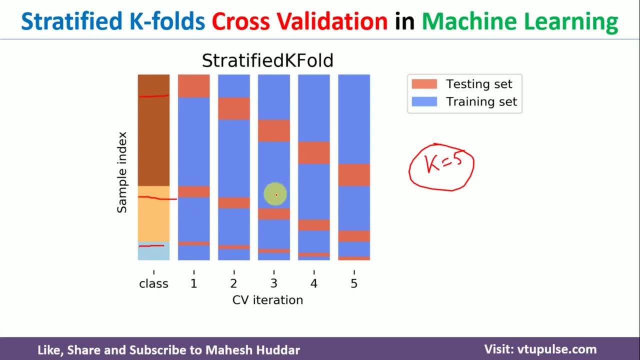 and so on. So if you do this particular thing, what happens is in each and every iteration we will get equal representation from each and every class of that particular data. So there will not be a bias, or you can say that the model will not go into a overfitting state in this. 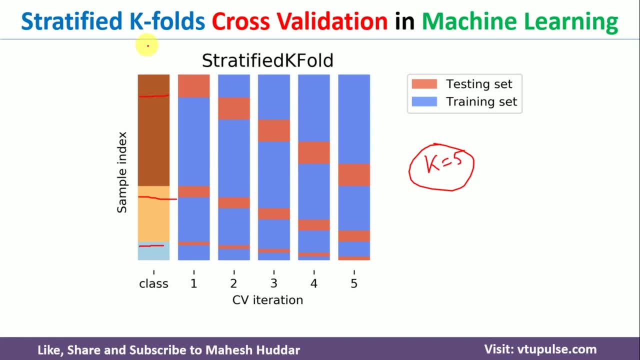 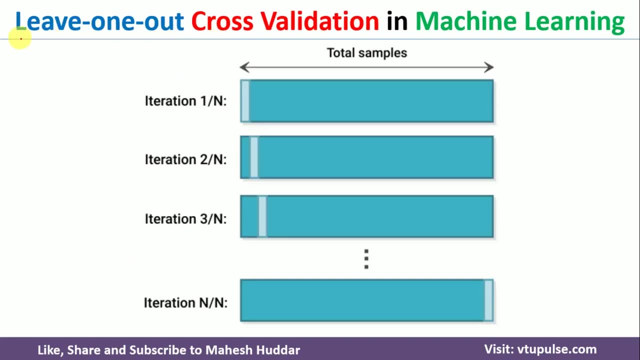 case. So this is how we can avoid the disadvantage of k-fold cross-validation: by considering the equal representation of each and every class. that is done with the help of stratified k-fold cross-validation here. Now coming back to the one more type of cross-validation that is called as leave-one-out. 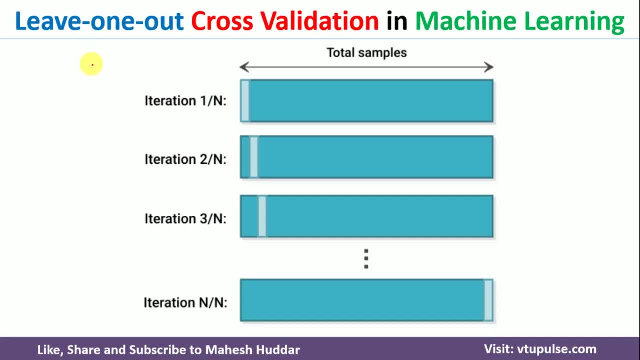 cross-validation. This is the extreme case of we can say that k-fold cross-validation, because in k-fold cross-validation we will divide our data into k-folds. For example, if we have k is equivalent to 10, we will divide that particular data into 10 groups. 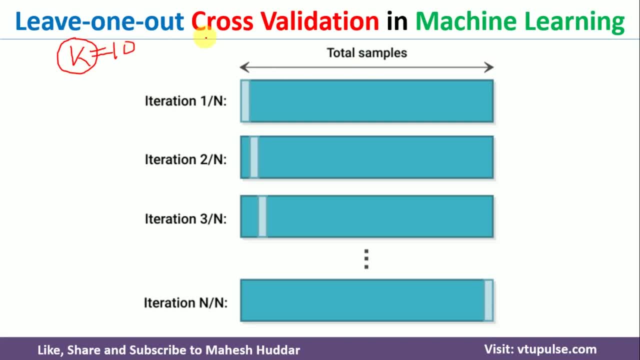 and then we will train it 10 times over there In leave-one-out cross-validation. what we do is we will consider one example for testing, remaining n minus 1 example for the train. The same thing will be done in each and every iteration. For example, if we have n number. 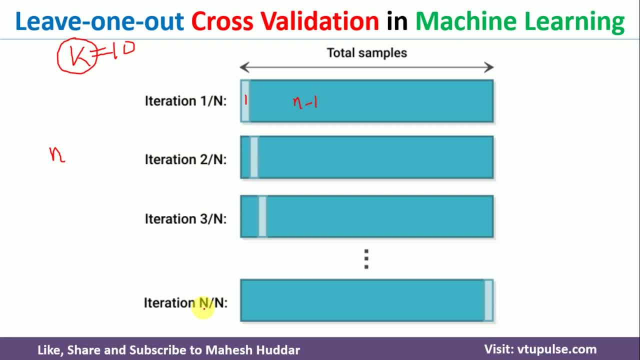 of examples. we will have n iterations over here. For example, let us say that we have some 100 examples. One example is used for testing and 99 will be used for training in the first iteration, and the same thing will be done 100 times over here. This kind of 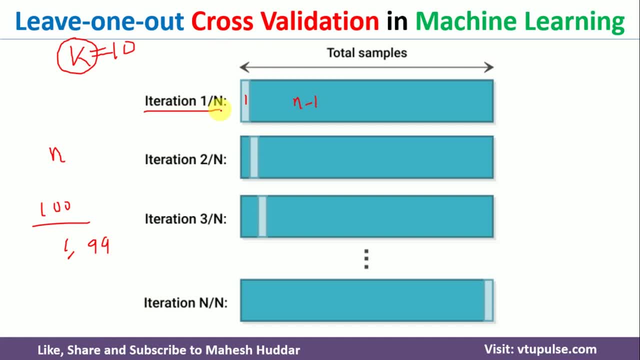 the cross-validation technique is not usually used in real world because it will take a lot of time to train. If we have 1000 or 10,000 number of examples, we have to train our model that many number of times. That is not usually feasible in real world. So we do not use this particular. 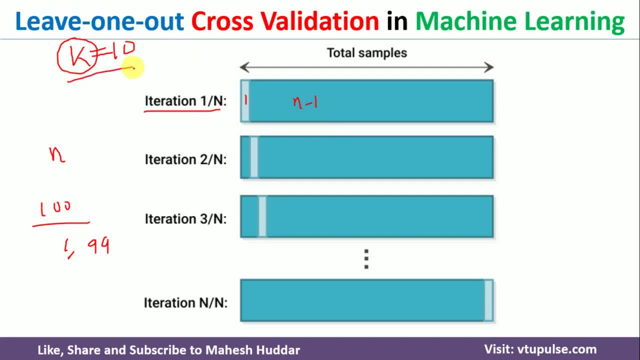 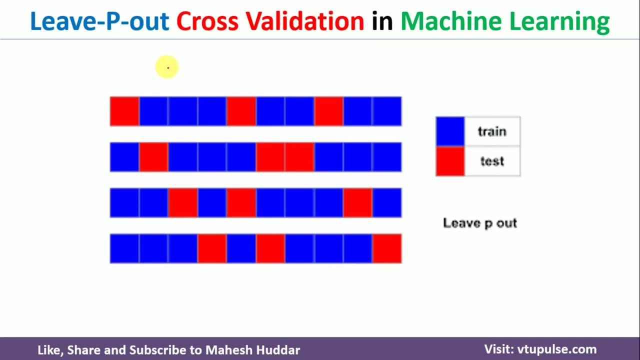 leave-one-out cross-validation. We usually go with something called as a k-fold cross-validation over here. Coming back to the last cross-validation technique, that is called as leave-p-out cross-validation. In this case, rather than going with one example for testing in each iteration, we will go 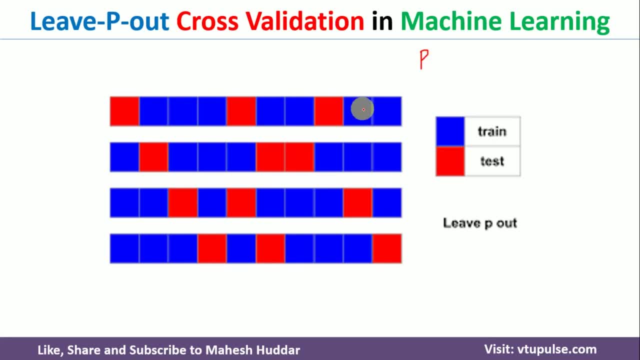 with the p example for testing in each iteration. That is the one thing, and another thing over here is these p examples. For example, let us say that p is equivalent to 3, that is, 3 examples will be selected randomly in each and every iteration. In the first iteration these 3 examples are considered for testing. 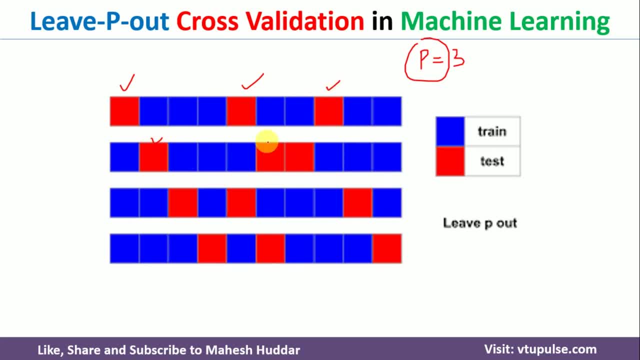 and remaining are considered for training. here, The second iteration, these 3 are considered for testing, remaining are considered for testing And if you look at this particular third one, one example which is considered for testing, which is already considered for testing in the first iteration, This is, this will happen because we are going to consider 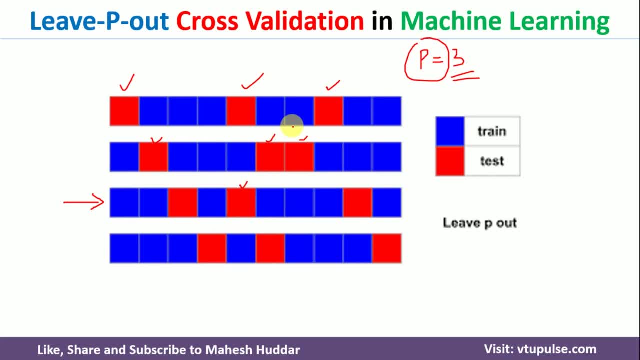 these particular 3 examples randomly. There is a possibility that the same example which was considered in the previous iteration will be considered for testing in the next iteration also. So in this video I have discussed what is the cross-validation, why cross-validation? 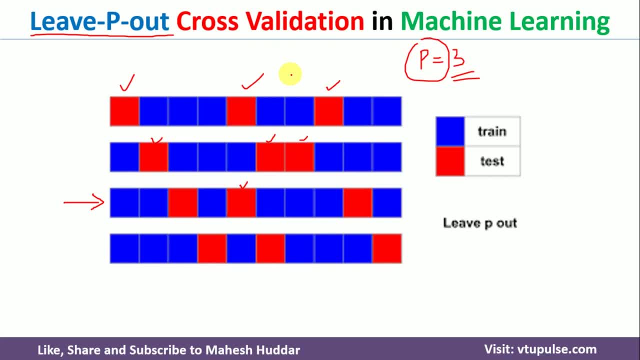 is required and what are the different cross-validation techniques. In the next video I will discuss how can we implement these particular cross-validation techniques. In the next video, I will discuss how can we implement these particular cross-validation techniques in the future python. i will put the link for that video in the description below. do follow that particular video. 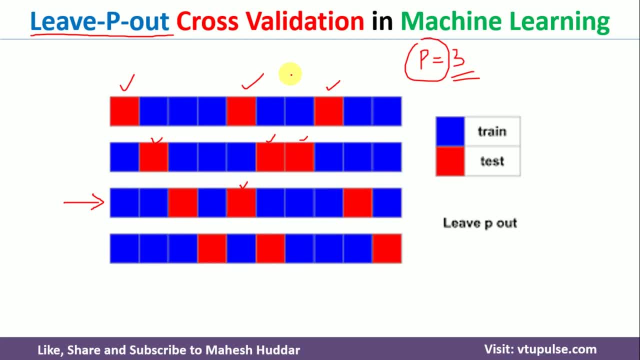 to understand how can we implement cross validation in python for building any machine learning models. i hope the concept is clear. if you like the video, do like and share with your friends. press the subscribe button for more videos. press the bell icon for regular updates. thank you for watching.